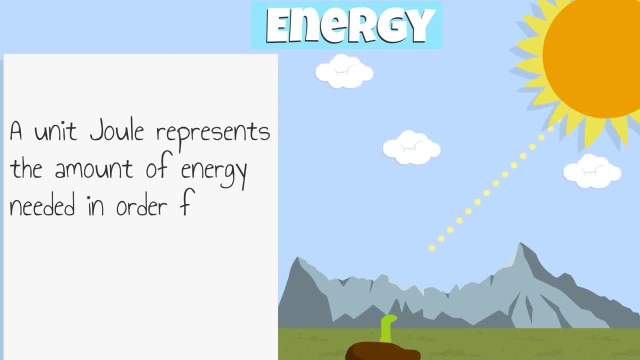 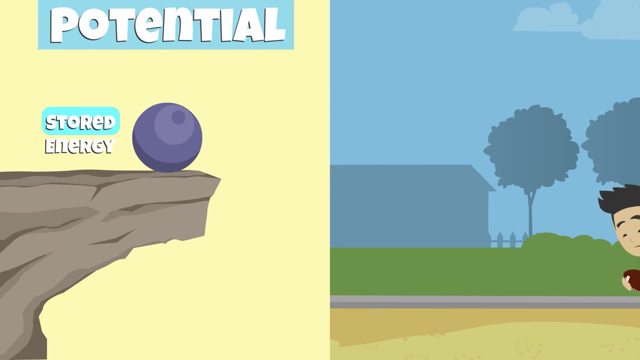 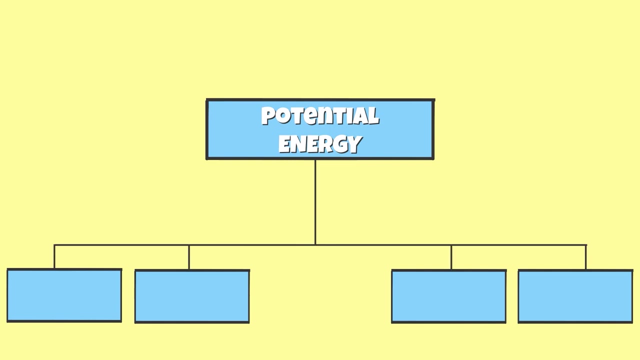 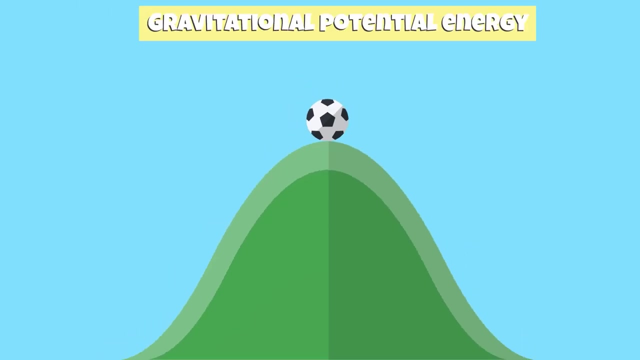 A unit joule represents the amount of energy needed in order for change to take place within a system. We define potential energy as stored energy, While kinetic energy is energy that is in motion. There are four types of potential energy: Gravitational potential energy, such as a child on a slide, a ball at the top of a hill or a hammer that is raised. 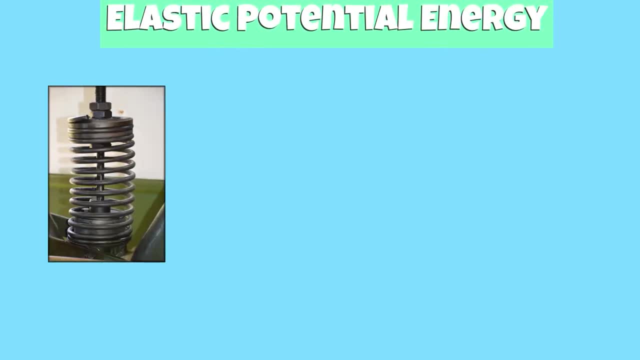 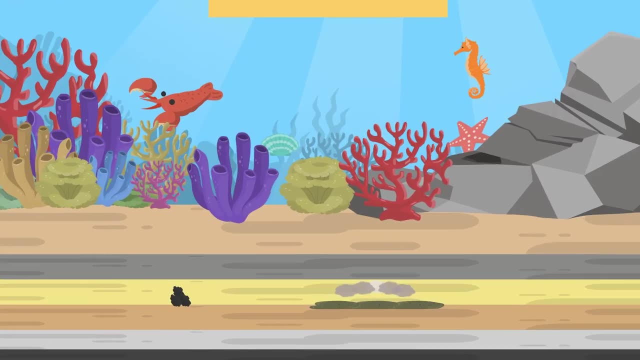 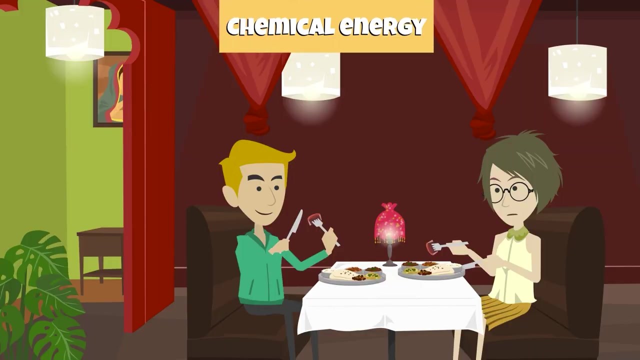 Elastic potential energy, such as a stretched spring or rubber band and a stretched bow. There's chemical energy: stored energy found in fossil fuels, Sunlight captured by plants, energy stored within a battery or energy stored in calories in the food that we eat. There's also nuclear energy. 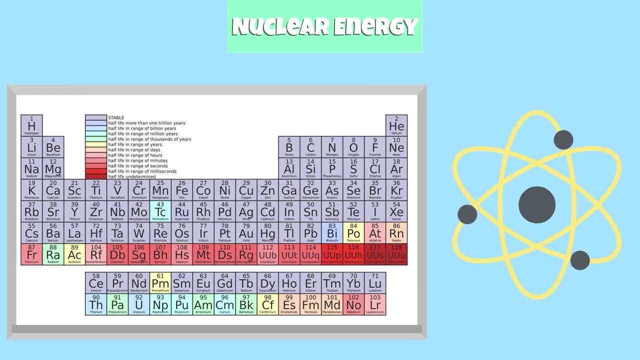 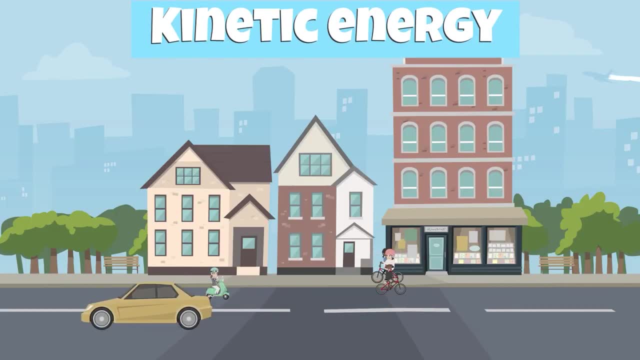 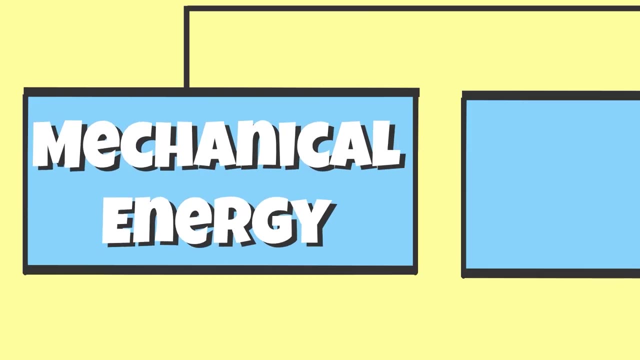 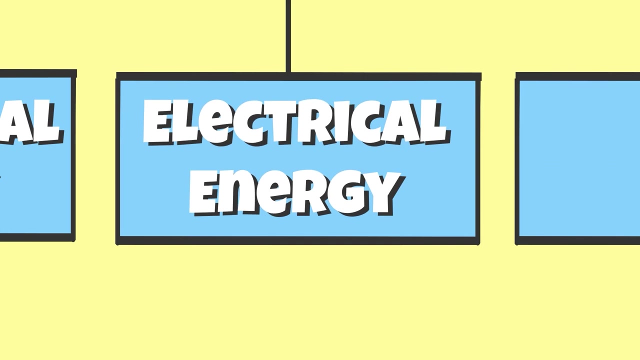 Potential energy stored in the nucleus of an atom. These are all examples of stored energy. Kinetic energy is energy that is in motion or that involves movement. Some types of kinetic energy are: mechanical energy, Such as cycling, riding a skateboard and driving a car. Electrical energy: the movement of electrically charged particles within a closed circuit that powers electronic devices. 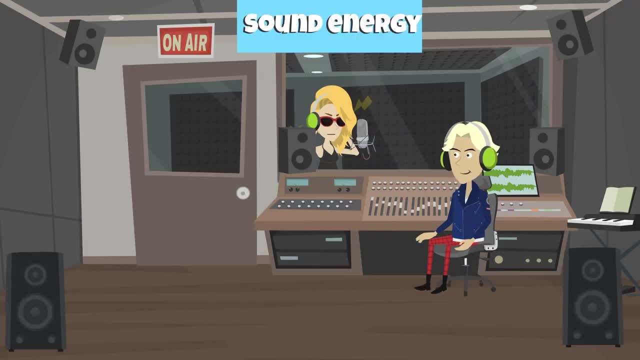 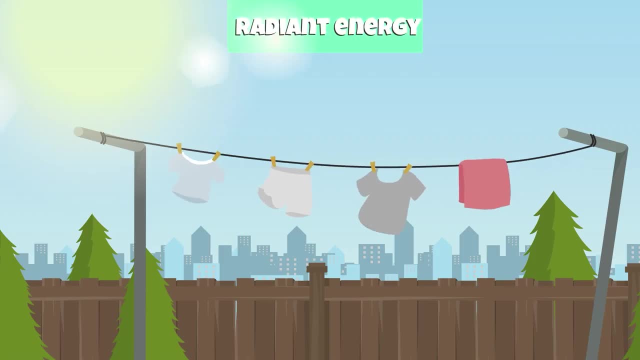 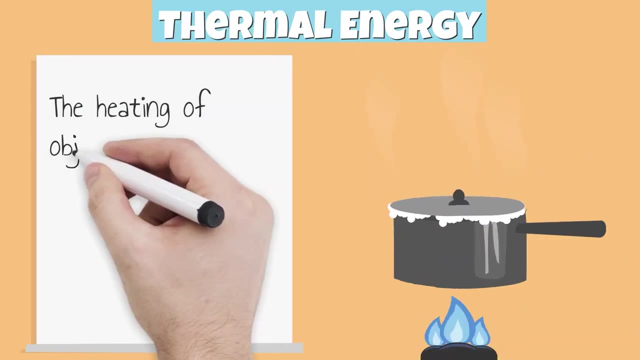 sound energy- energy that moves and travels in sound waves, such as a speaker blaring. radiant energy- the electromagnetic energy that travels through sunlight, radio waves and x-rays. and thermal energy- The heating of objects that cause atoms and molecules to vibrate, move rapidly and collide with each other. 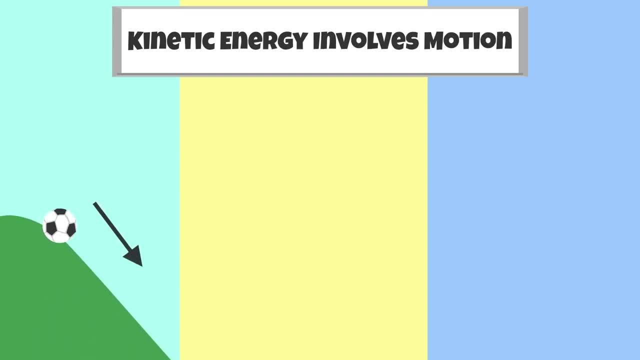 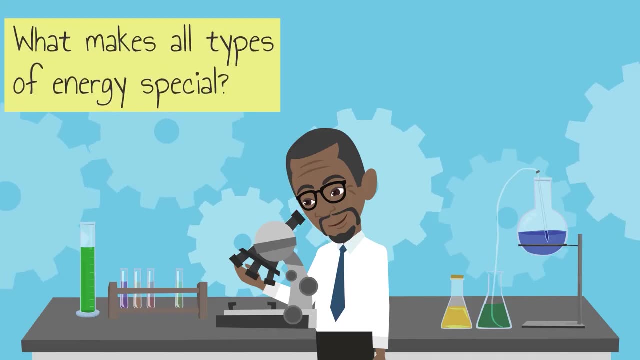 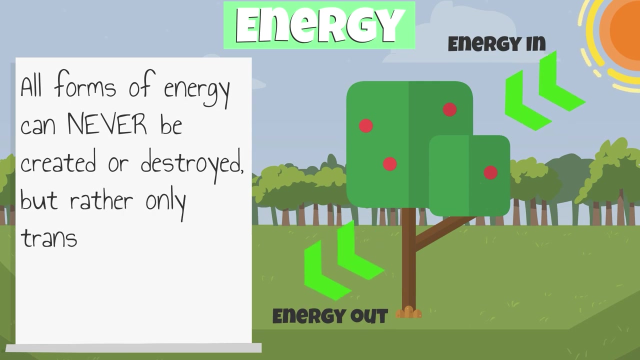 Kinetic energy involves motion, such as a ball rolling down a hill, a book falling from a table or throwing a ball. So what makes all types of energy special? All forms of energy can never be created or destroyed, But rather only transferred between an object or a system. 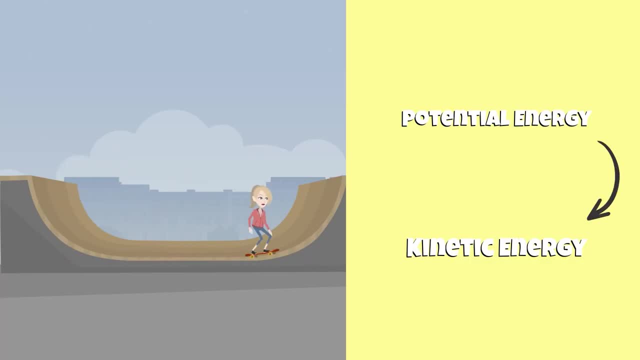 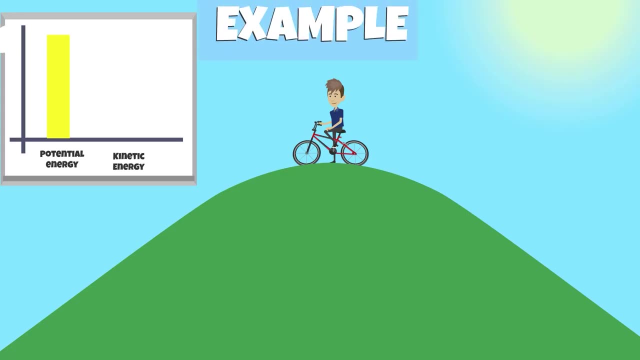 Potential energy can transform into kinetic energy, and kinetic energy can also change into potential energy. For example, if you're to be at the top of a hill on a bicycle, You would have the greatest amount of potential energy, or energy that is stored, The minute you start to go down the hill. the stored energy is transformed to kinetic energy, or energy of movement.